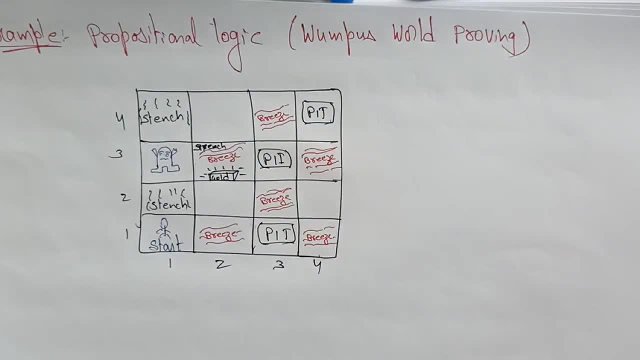 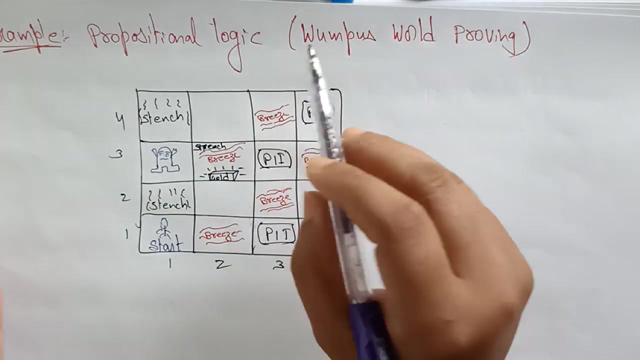 Hi students, welcome back Now. coming to the example of the propositional logic, In the previous video I explained one of the logical representation is the propositional logic. So in this exam, to explain this propositional logic, I'm using one of the famous problem, that is, a Wempus word problem. 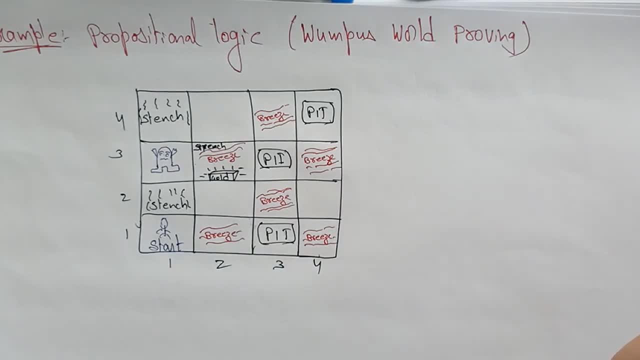 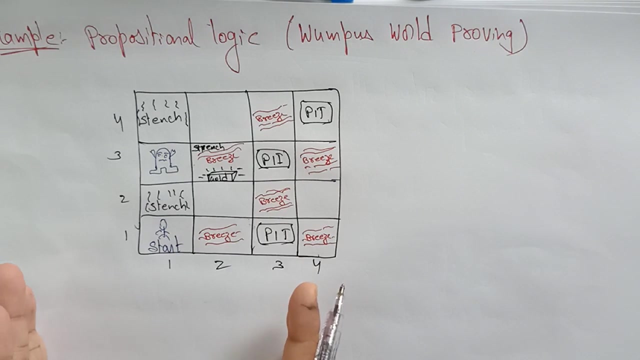 Okay, Wempus word problem. So before applying the propositional logics, I want to explain you what is this Wempus word proving, And you can always call it as a Wempus word problem also. Okay, so this is a problem. I'll explain the problem first. Later I'll apply how the propositional logic is used to solve this Wempus word problem. Okay, let's start. Come on. 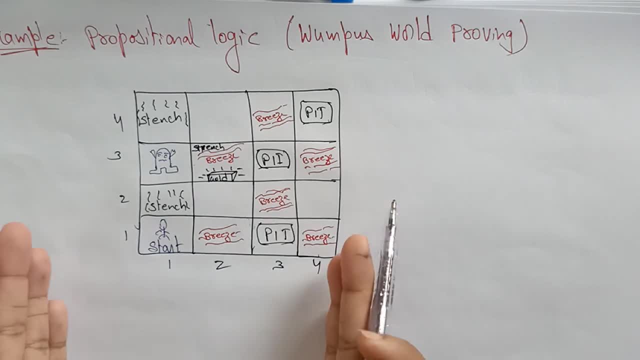 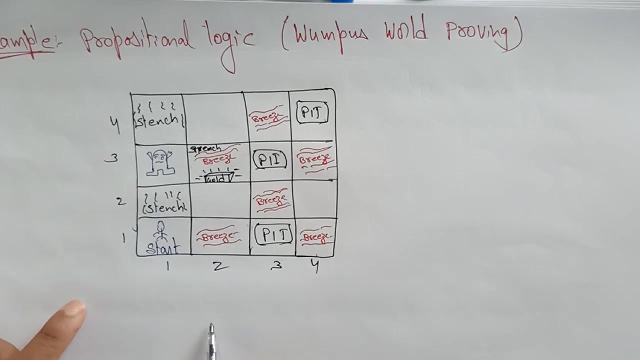 So here I have taken, First let me explain you- Wempus word problem. What is this, the diagram I have written here, And what are the conditions or the some components which can help the agent to navigate the cave? Okay, and some rules. So first I'll explain all these rules. So here this is. let me take this as an agent. here An agent is present. Let's take anyone, Okay, any artificial intelligent is present. That is the agent here. So the agent always starts in the field one one. Okay, it's just starts in the field one comma. 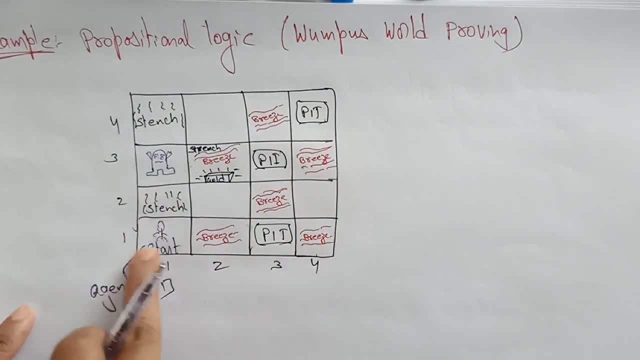 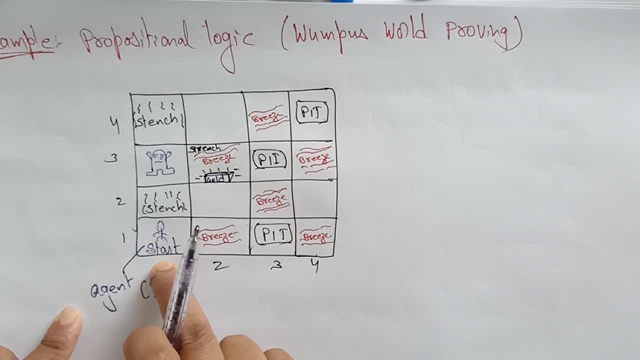 Gold is there. So the task of this agent is to find the gold. Okay, and return to the field again. he has to find that gold and he has to return back to this position, one one, and he has to clip out of the cave. So this is completely a cave, a cave consisting of all these rooms. In each room, something is there. In one of the room, a gold is there. The agent has to find out that gold by crossing all these rooms. Okay, he has to find the gold and he has to find the gold. 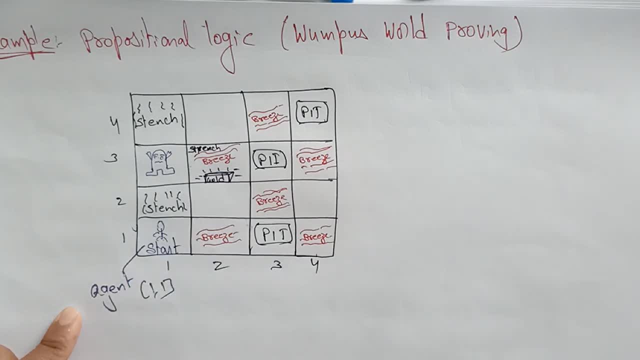 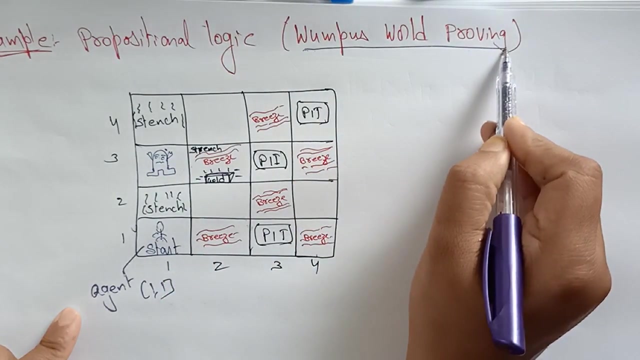 Again return back to this position and jump from the cave. Okay, he has to get out from the cave. Okay, without falling into pits. So here some pits are there without falling into pits, and vampas and or eaten by the vampas. So here one vampas is there, Okay, which is like a monster. you can call it as a monster, Okay, so this is a vampas word problem, So that's why we call it as a vampas. It's just like a monster means this person cannot enter. 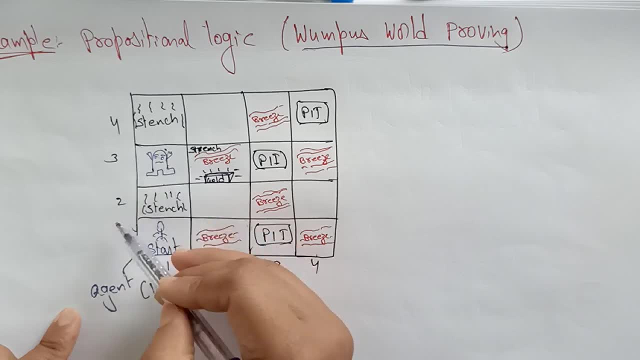 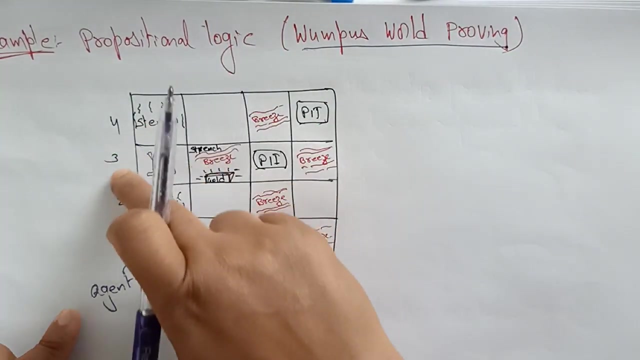 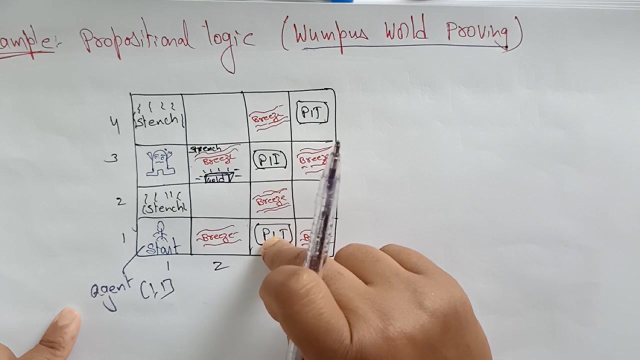 into this room. So if he enter into room he can be eaten by the vampas, Okay, or the person can shoot that vampas. also, there is a chance, there is a condition, Okay. so the pit and vampas here are the static. they cannot be moved. The pits will be fixed and the vampas is always stay in this room only, Okay. and the pits, Okay, these are will be in this position, only, they cannot move. here. pit rooms which are bottomless. pit means you know that it's just a dig, it which is 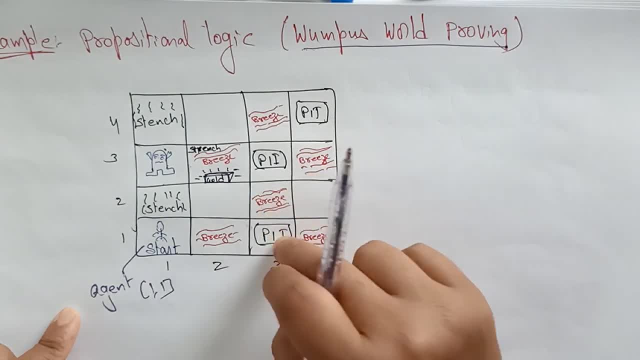 having the bottomless If suppose if agent enter into that he fall into pit and then he will be struck in that forever. He will stuck in that pit forever. He can't get out, get out from that. So we he has to take care without falling into the pit. Okay, and this is a. the agent has a single arrow. You remember that he's having only a single arrow here. Now let's see there are some components which can help the agent to navigate the cave. So I said here: 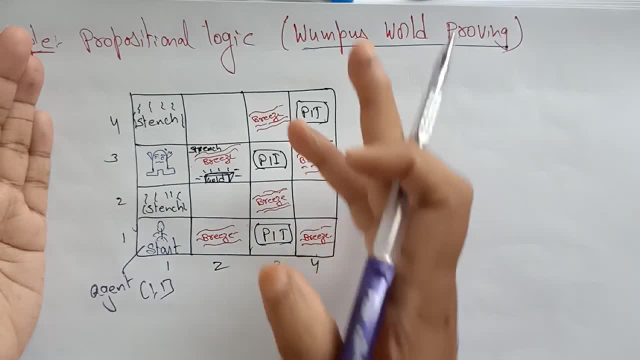 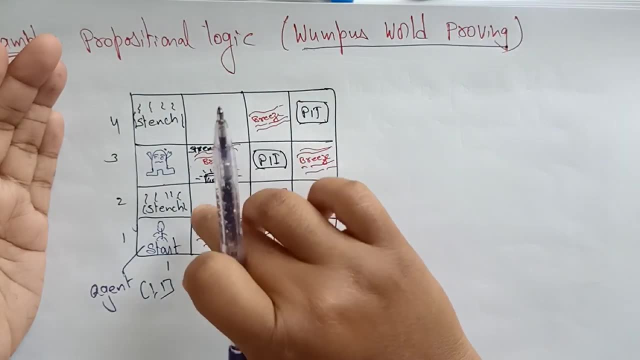 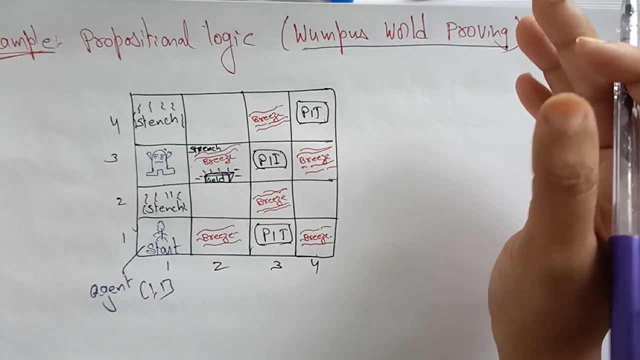 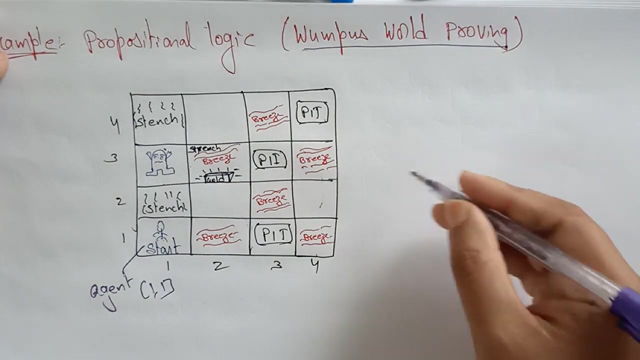 there are total so many rooms are there. Okay, so total 16 rooms are there. four by four, matrix 16 rooms are there in each room. Some pits are there, some breeze is there and stench is there, and vampas is there, and the person and the gold is there, all these things. Now let me, with the help of those conditions, the person can navigate into each and every room. So what does this conditions? Let's see, The first condition is the rooms adjacent. to write me right. 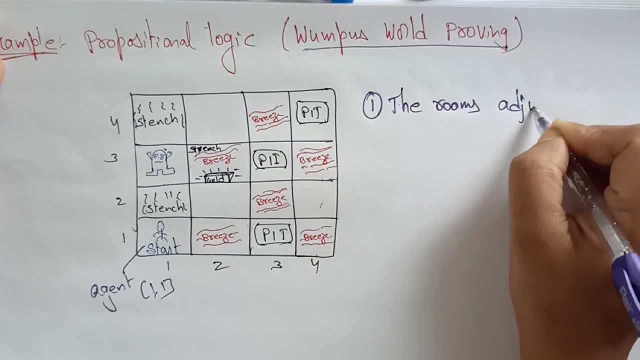 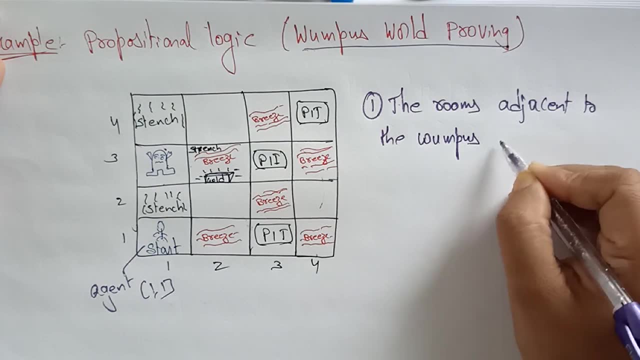 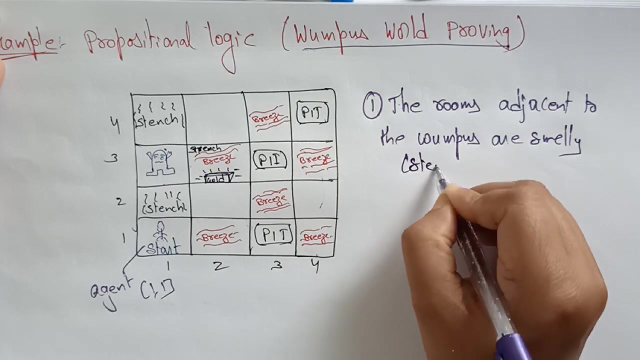 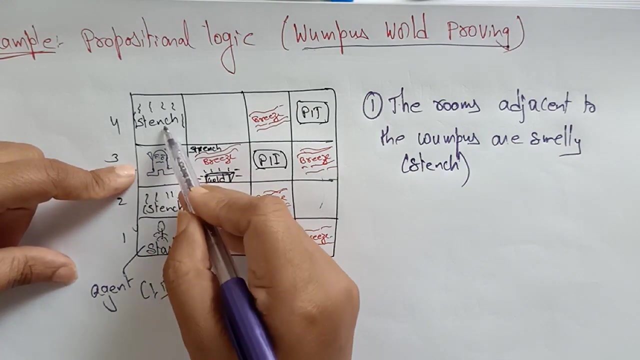 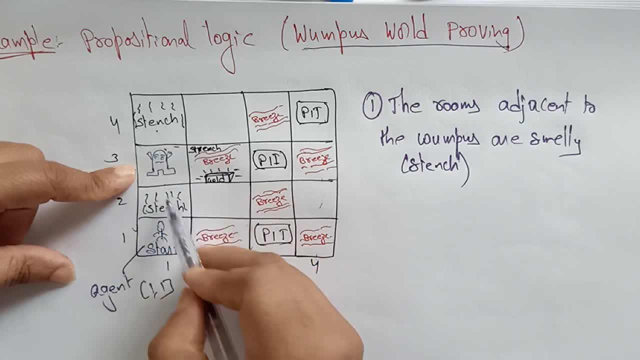 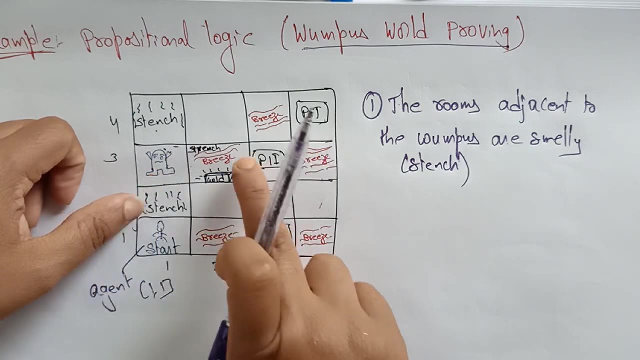 Okay, that means it is something smelly. Okay, that's why I keep in the symbols like this: a smelly, the smell. Suppose a person enter into the room He can recognize the adjacent room is the vampas because it is smelly. It suppose the person enter into this room He can recognize the adjacent room is having a stench. Okay, these are the adjacent rooms to that person. There is a stench because there is a vampas here. 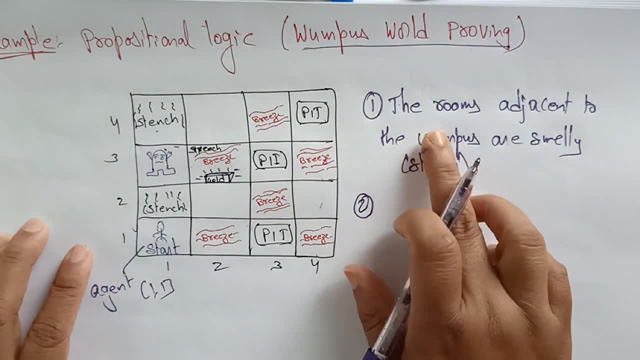 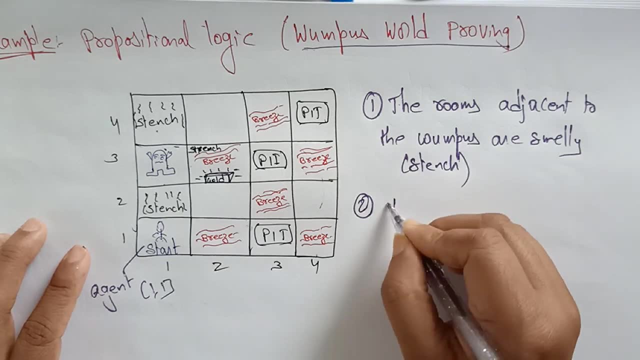 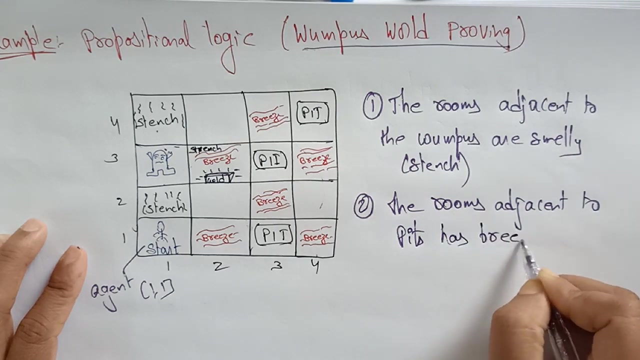 That's why it has become smelly. That is the first condition. So remember that The rooms adjacent to the wampus are smelly. Second condition: The rooms adjacent to pits has breeze, So let us assume the rooms Here. it is there. 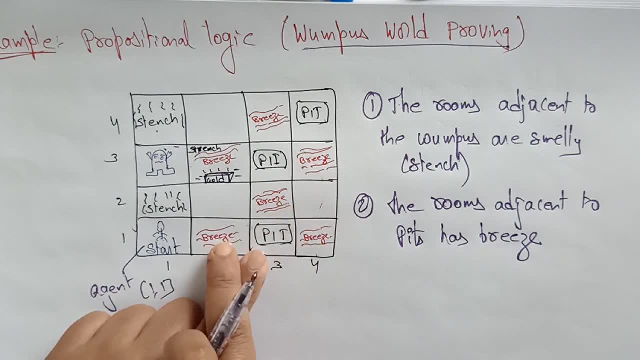 The rooms adjacent to the pits has breeze. See here, The adjacent rooms is having breeze. The pit adjacent rooms is having the breeze. The pit adjacent rooms are having the breeze. That means whenever the agent enter into that breeze room, So then he will perceive the breeze. 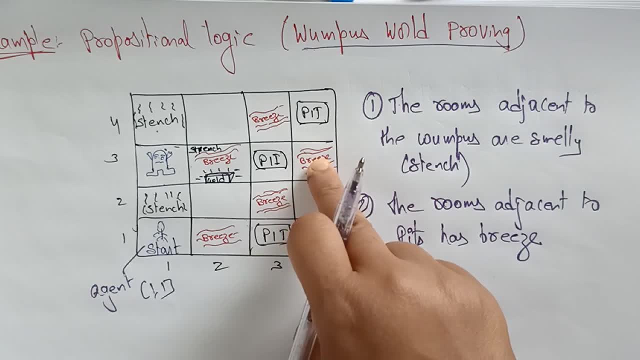 Okay, He is saying that. okay, here the breeze is coming. That means the adjacent room of this breeze is a pit. The adjacent room of this breeze is a pit. Okay, The adjacent room of this breeze is a pit. So that is one condition. 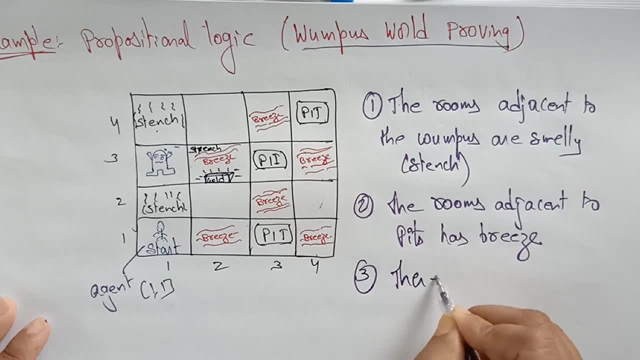 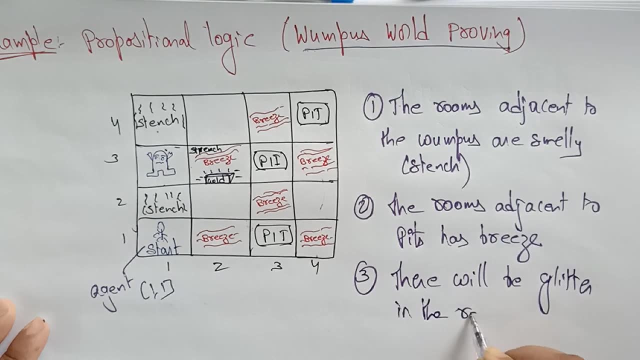 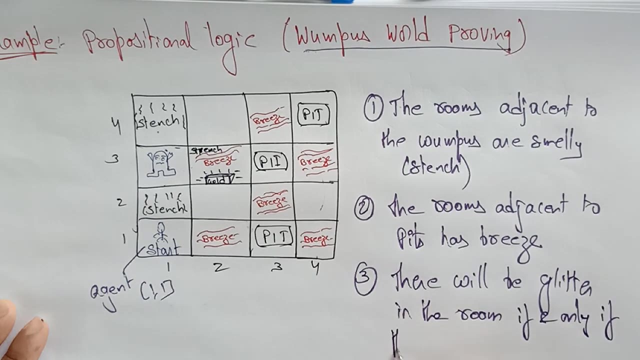 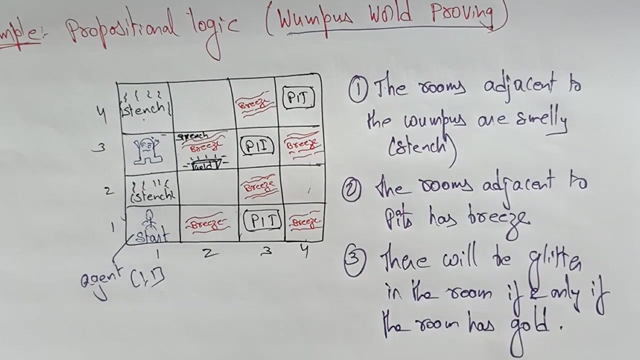 And next there will be a glitter. There will be glitter in the room. In the room If, and only if the room has gold, If and only if the room has gold. Okay, So there will be a glitter. So if the room 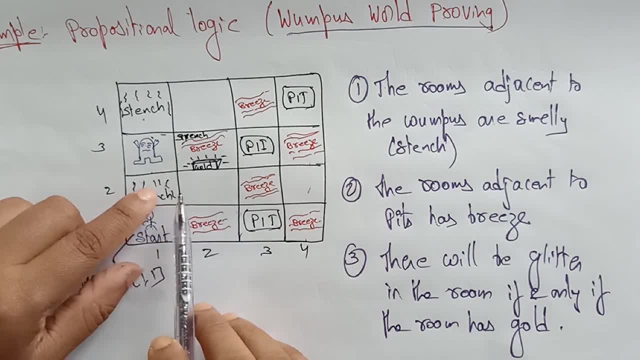 If, and only if, the room has a gold. So if suppose if the person is standing here There will be a glittering. So suppose if the glittering is coming means that the room is having the gold And next the wampus can be killed by the agent. 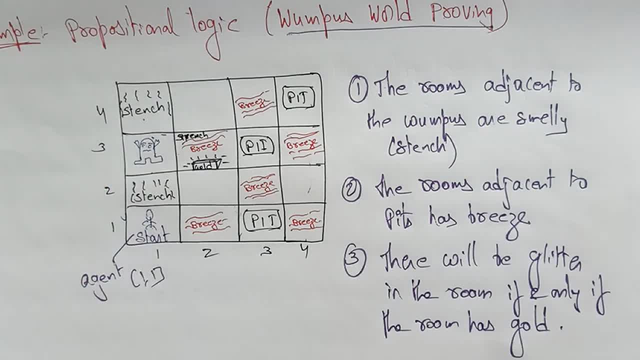 If the agent is facing to it directly And the wampus will emit a horrible scream also. So remember that the wampus is sometimes it is used to roar, like anything. Okay, It is a horrible scream. is there Which can be heard anywhere in the cave? 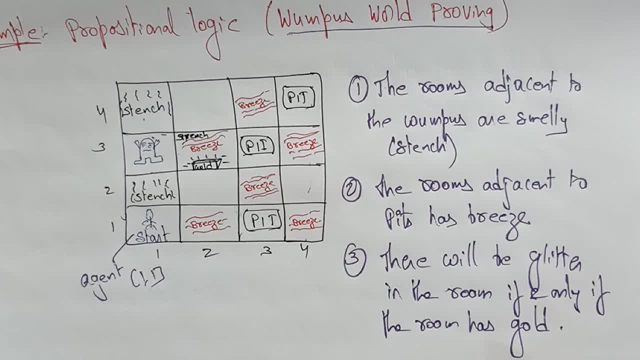 Anywhere in the cave, it will be horrible. So, with the help of the sound also, he can recognize that the wampus is in which room? also, Okay, So these are the conditions. With the help of this condition, the agent is moving towards this rooms to identify where the gold is present. 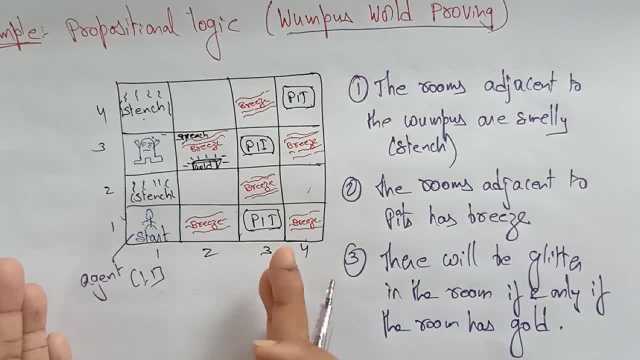 So here the agent can move to the left turn or right turn, or move forward or backward, or grab, release or shoot, Anything he can do. That is the agent can do, Okay. And here the sensors. The agent can sense, stench, smell. 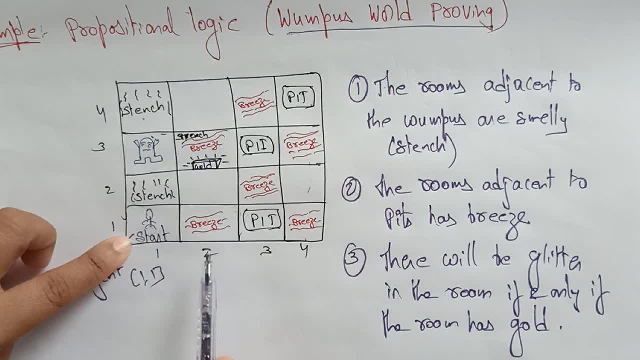 That is a bad smell. he can sense. He can sense the breeze also, And he can sense the glitter also. That is the gold. Okay, Sensors, These are the sensors, Let me write those point: Activators in this artificial intelligence. 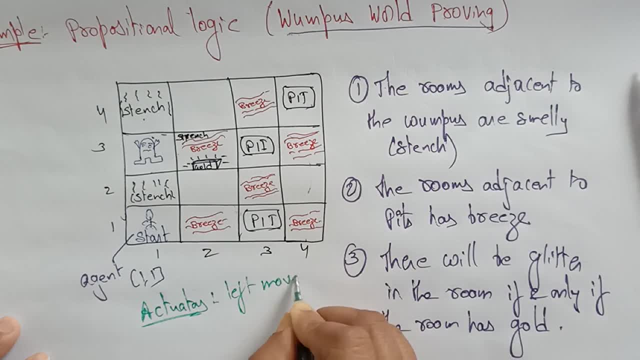 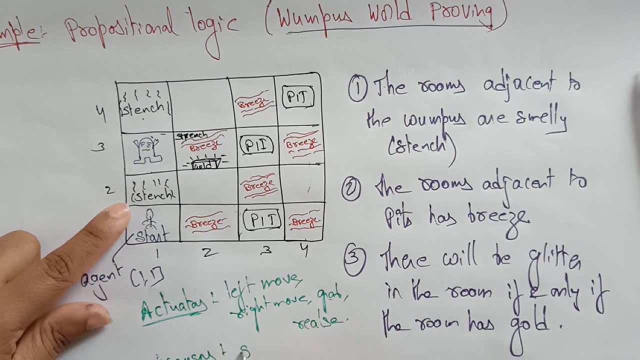 Activators are the left move, right move, Left move, right move or grab forward, release, Shoot or these or the activators And where does the sensors are? He can sense the stench smell and breeze smell, glitter smell. 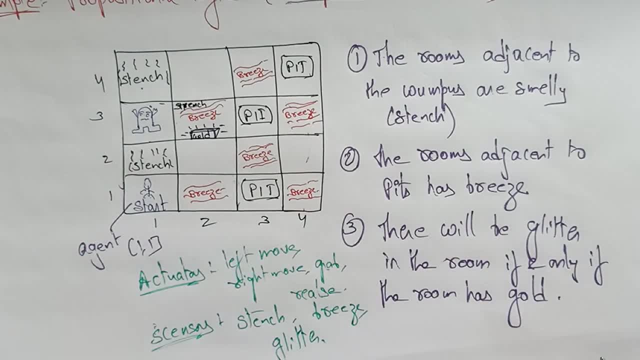 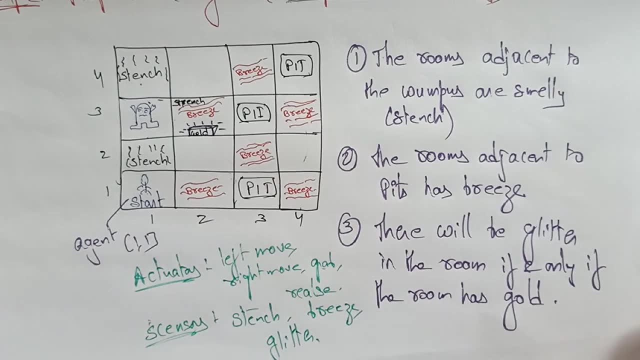 If the gold is there, he can sense the glitter. He can observe the glitter, Okay, And the scream also, the sound also, he can be sense, Okay. Now let's explore how the agent, The agent- can reach the gold And take the gold and he can jump out of the cave.